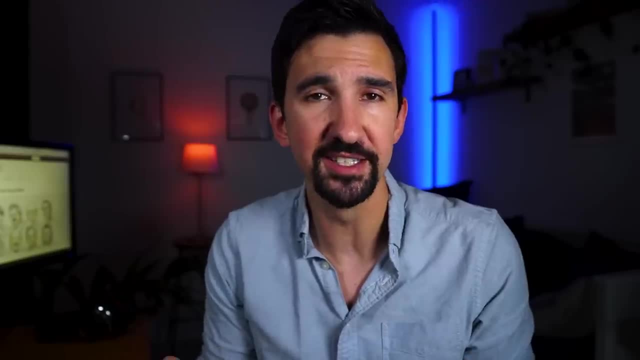 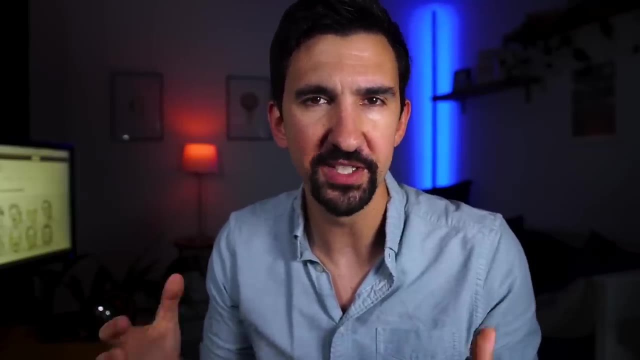 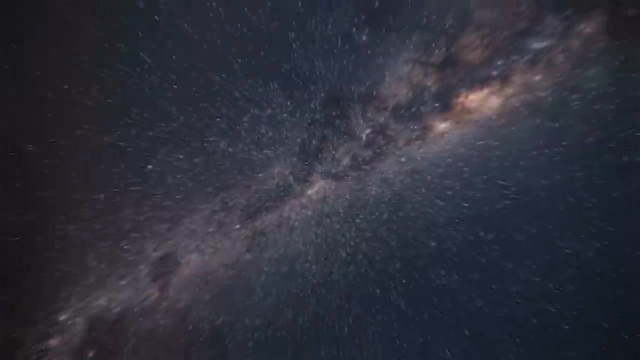 being confused and how ultimately Einstein was proven wrong, which doesn't really happen all that often. That idea of locally real is made up of two concepts. Locality is the idea that things are only affected by their local environment. You can't flick a switch in. 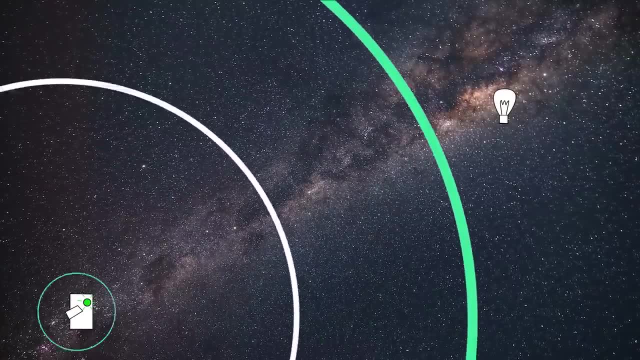 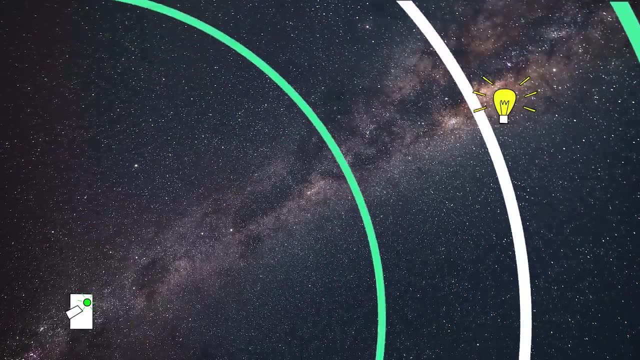 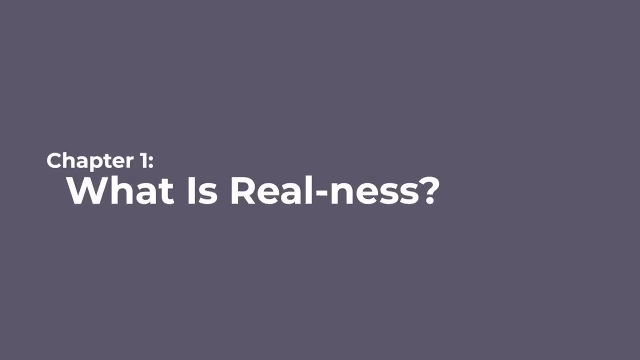 another galaxy hundreds of light years away, and instantly see the results here, because nothing, not even information, can travel faster than light. Realness, though, is much harder to explain, and that is the focus of the Nobel Prize. Let's start close to the beginning, around the 1930s, where there were two paradigms: 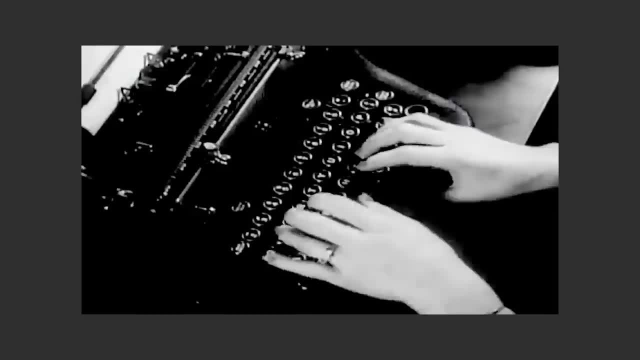 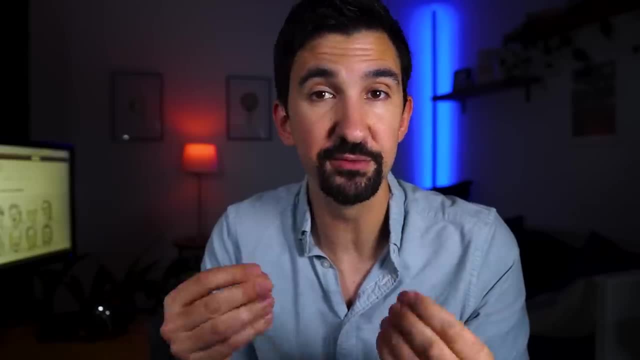 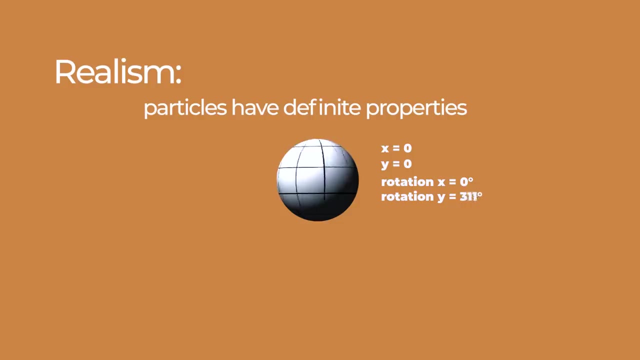 two ways of thinking about the physics of small things like particles, atoms, electrons, photons, etc. The view of Einstein and many others was that the universe is real, that particles, atoms and electrons have definite properties that are inherent to them, regardless of if they. 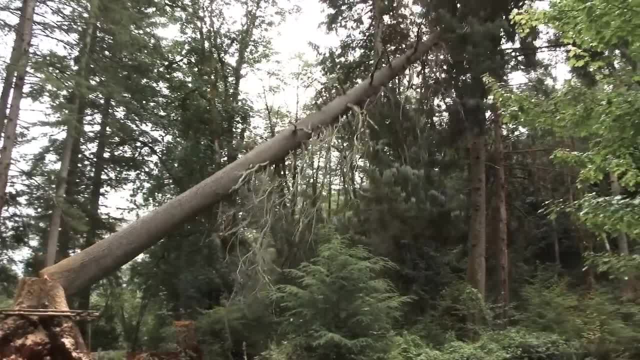 are being measured Essentially that if a tree falls into the water, it will fall into the water. If a tree falls into the water, it will fall into the water. If a tree falls into the water forest and no one is around to hear it, it does in fact make a noise. and then there was a counter. 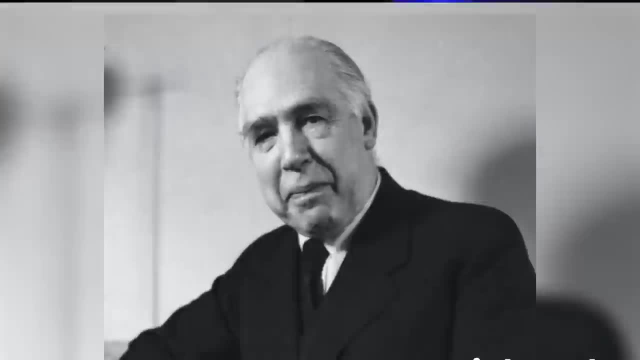 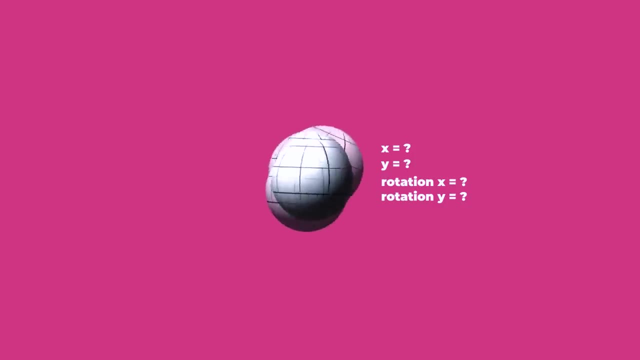 group, the anti-realists, championed by people like boar as well as many others, that particles have properties that haven't really made up their minds until you actually go out and measure them. that they exist in a wave function of possible states, and only when you actually take a measurement. 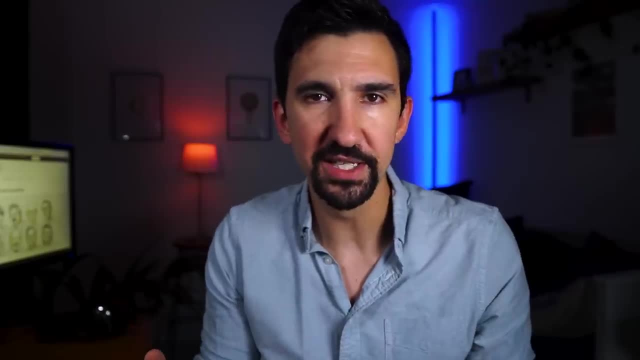 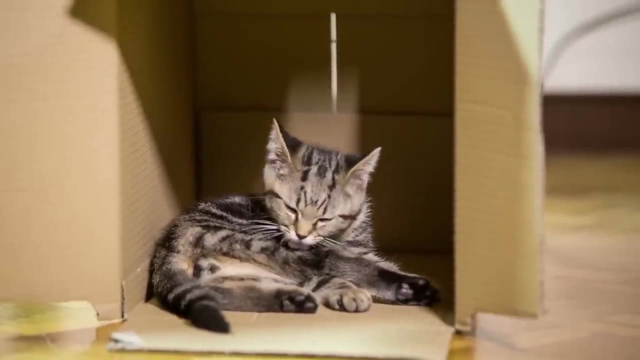 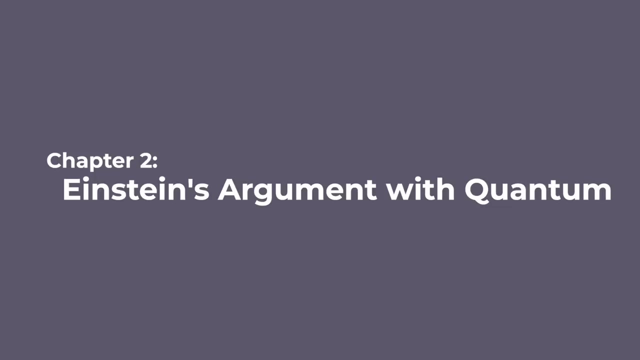 do they really make up their minds? the famous example here is that of schrodinger's cat that is both alive and dead until you look in the box and then, ultimately, you go to prison. this back and forth between boar and einstein culminated in a famous paper called the epr paper. 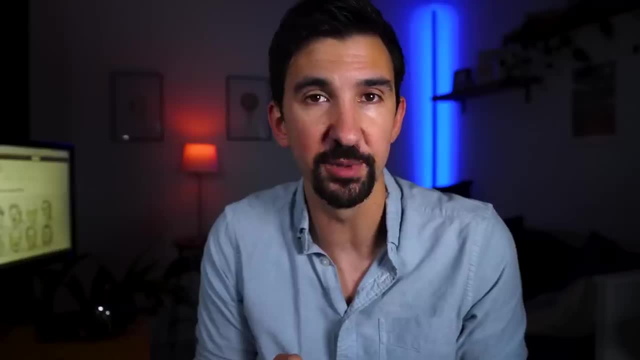 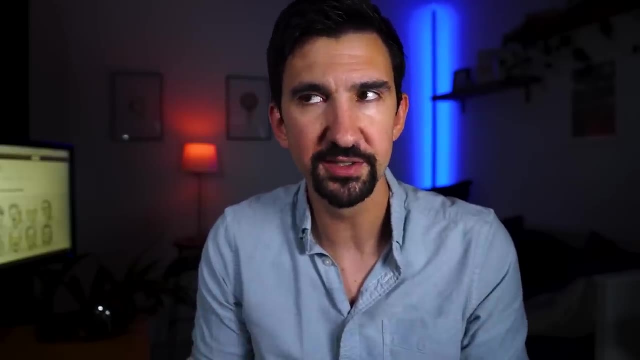 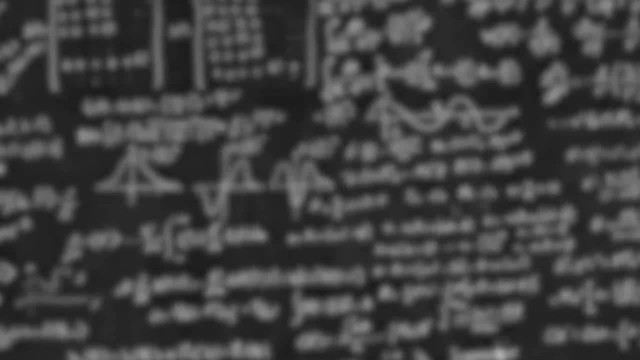 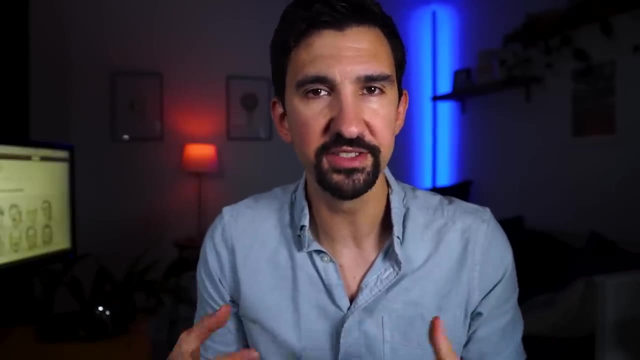 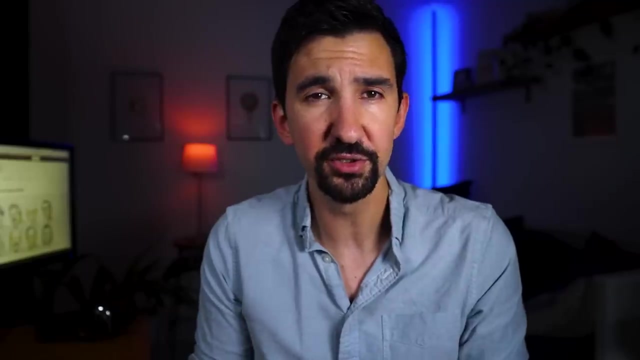 mechanics called entanglement that the property of two particles can be inherently related. their line of reasoning for their thought experiment started with: well, we know that energy is conserved. things don't suddenly start moving in a direction, unless someone or something pushes or pulls them. neither also do they suddenly start spinning, rotating, jumping up and down or doing anything else. 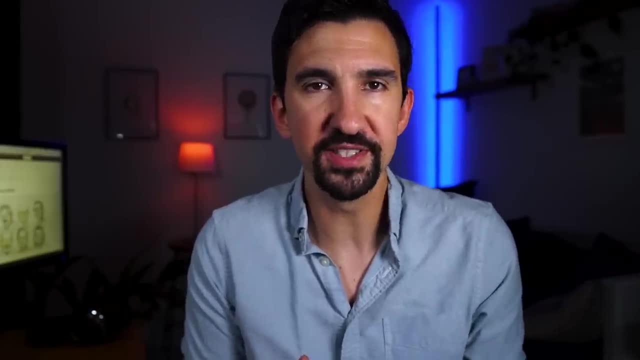 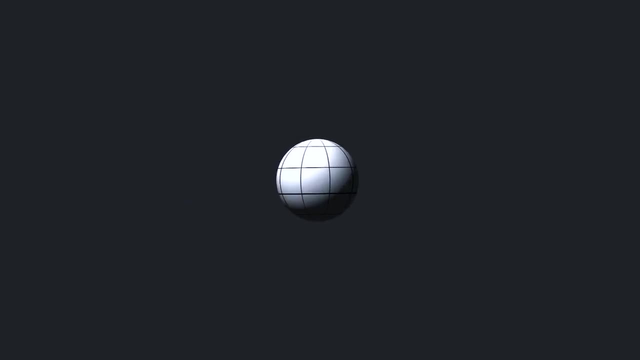 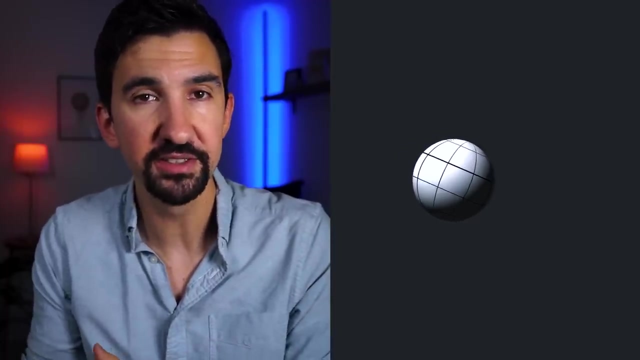 unless someone else is directly affecting them. number two: if we start with a small quantum mechanical particle that isn't spinning, moving or doing anything else, let's imagine that particle spontaneously breaks into two. if we look at one of those pieces it breaks into and find that it's moving to the right. 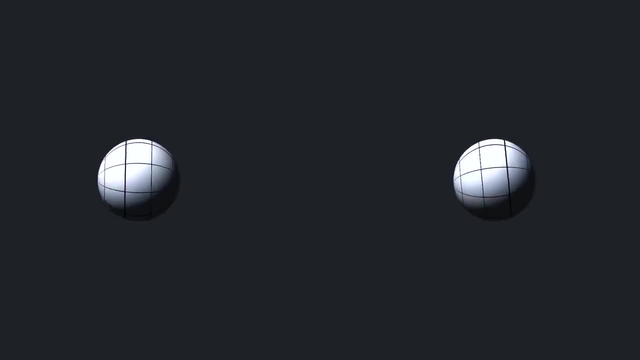 we know instantly that the other particle must be moving to the left to conserve momentum. or if we had looked at it and found that it was spinning one way, maybe clockwise, we would know instantly that the other particle must be spinning counterclockwise to conserve angular momentum. you've 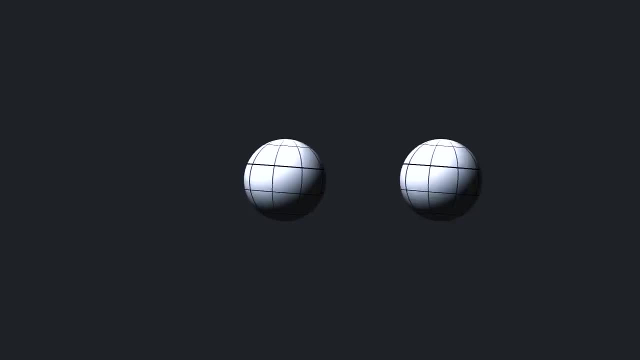 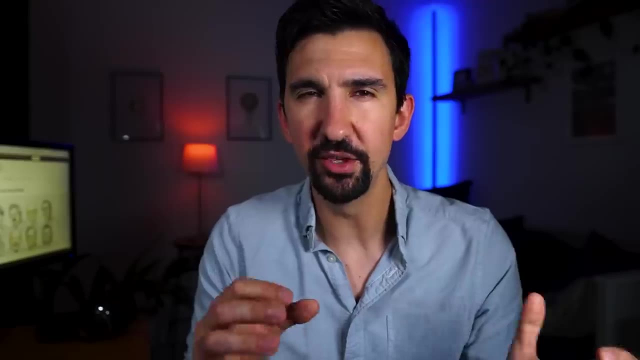 been confused. if you looked at this system and saw both particles suddenly moving to the right, your intuition would tell you that some outside force maybe must have hit them. or for the same reason, though maybe less intuitively, because most people don't think about angular momentum or spin. 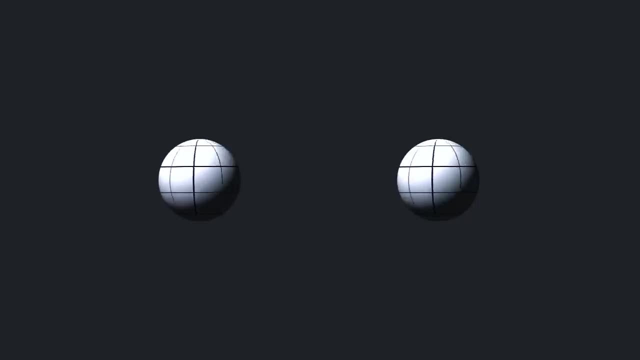 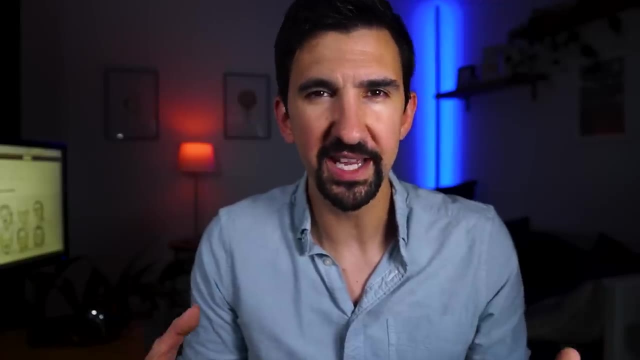 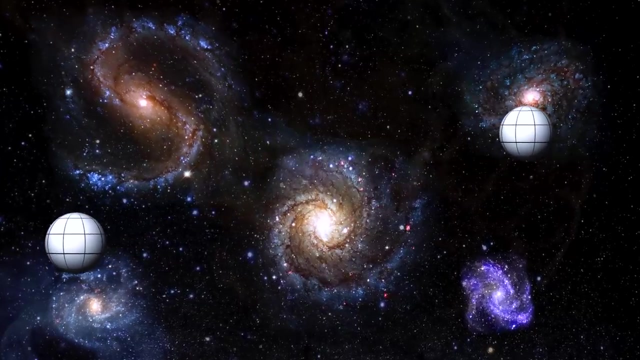 you'd be equally surprised if you saw both particles rotating in the same direction. you'd assume that something must have hit them and caused them both to start spinning. step three, quantum mechanics here says these states are impossible to know before you go out and measure them. If you separated these particles light years apart? 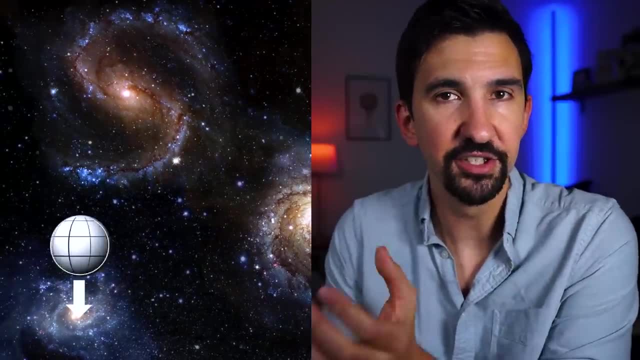 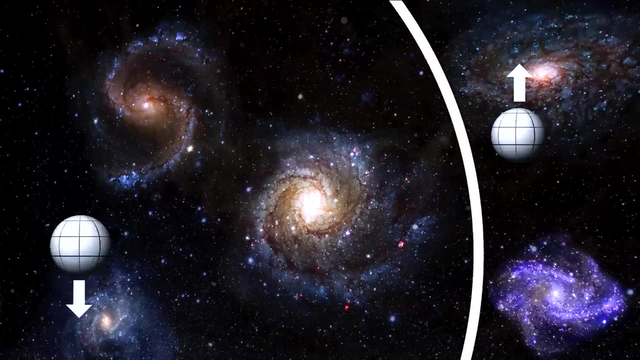 and measured one say, and found that it was spinning clockwise, you'd know instantly, even if that particle was a universe away, that its counterpart must be spinning counterclockwise. But how could this be, If they really only take on a definite value? 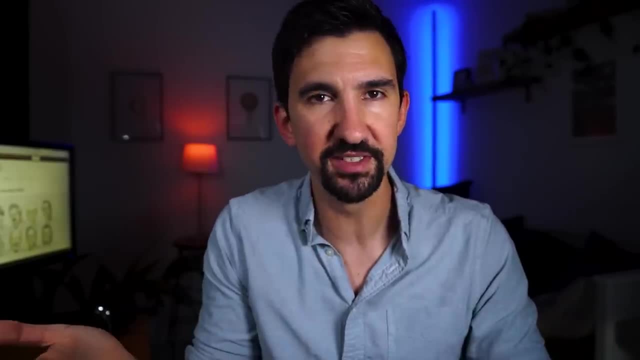 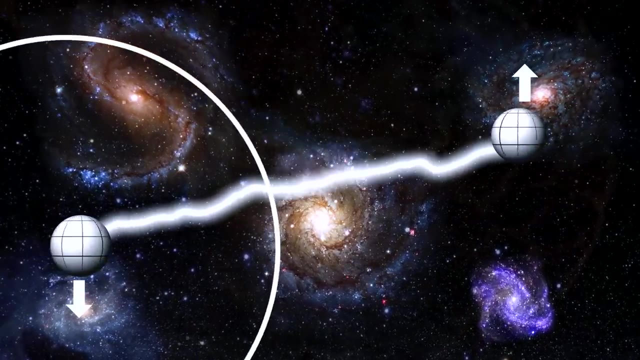 when you measure them, and the other one always needs to be the opposite of what you've measured, then the particle that you did measure would need to instantaneously communicate to its partner and tell it to adopt the opposite value permanently. Einstein argued that this was impossible. 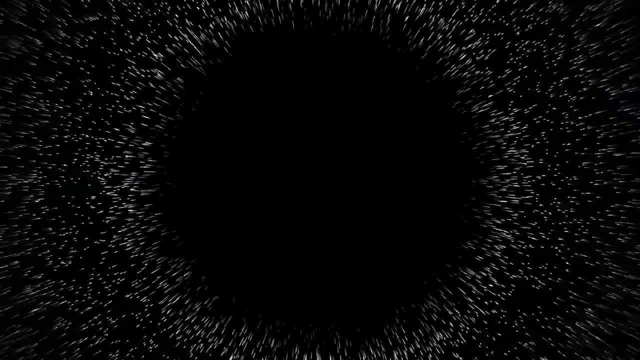 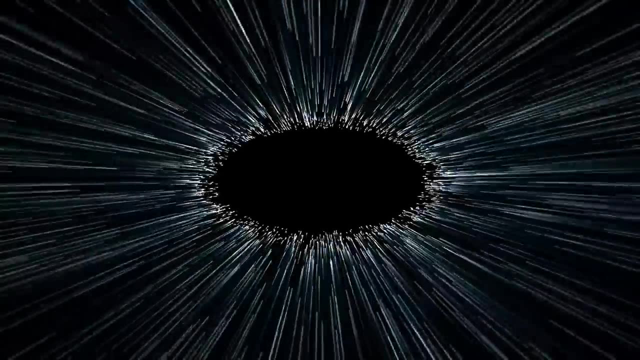 because it would have violated locality and meant that information had traveled instantly- faster than the speed of light- to tell the other particle to collapse its wave function and make up its mind which way it was spinning. Instead, he argued it must have made up his mind at the very beginning. 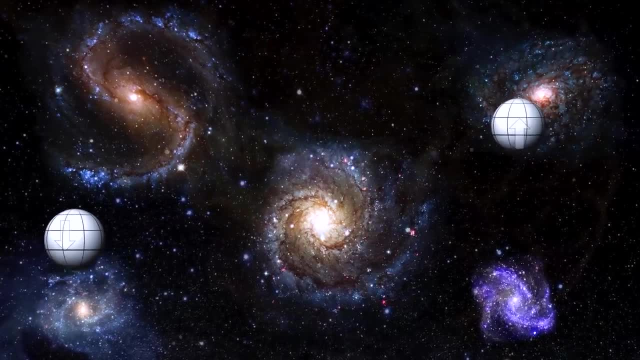 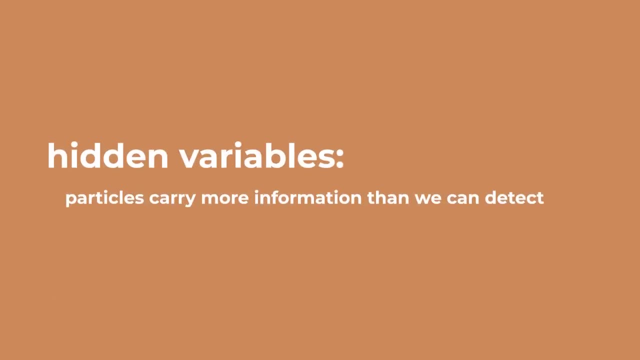 when it was created. We just didn't know it, or we weren't smart enough yet to find a good way of measuring it. He called this unknown knowledge hidden variables and said that this was the piece in quantum mechanics that was yet to be completed. 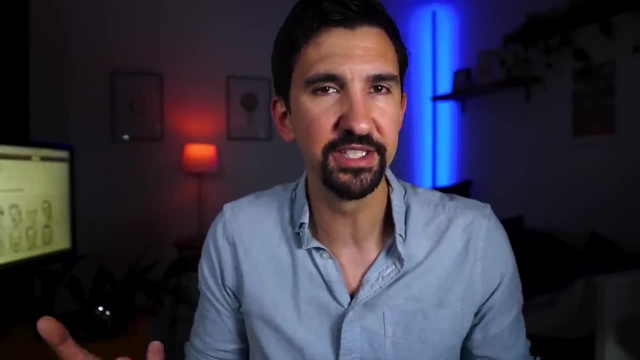 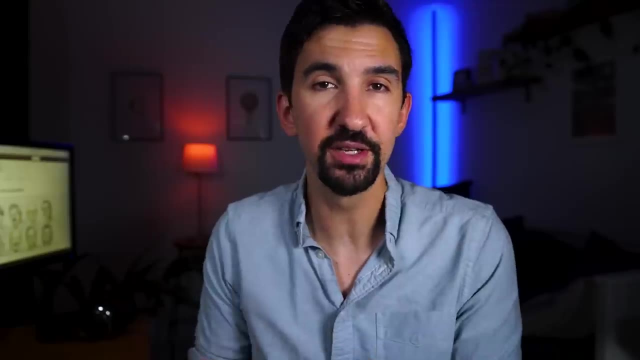 And for around 30 years physicists really kind of split into two groups. Either they sided with Einstein or they sided with Bohr, Mostly because no one had really come up with a good theoretical or experimental counter argument to Einstein's EPR paper. 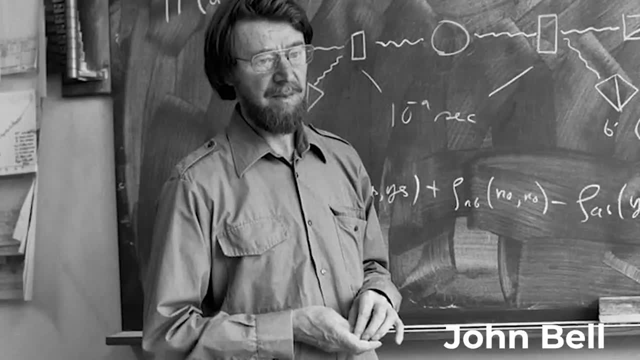 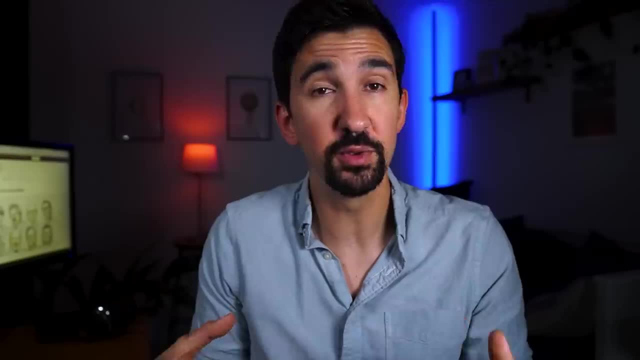 That was until about 1964, when John Bell, an Irish physicist on sabbatical from working at CERN, started to do some more theoretical work of his own. These works, which were later called Bell's theorem or Bell's inequalities, 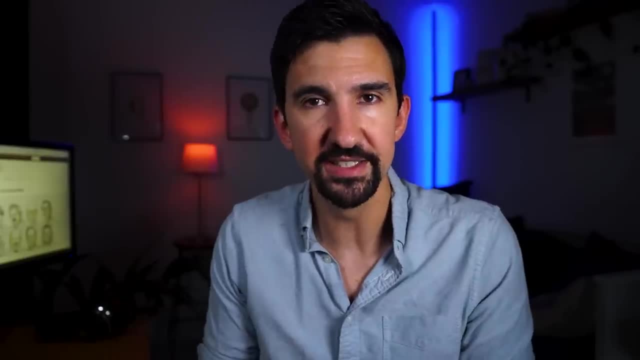 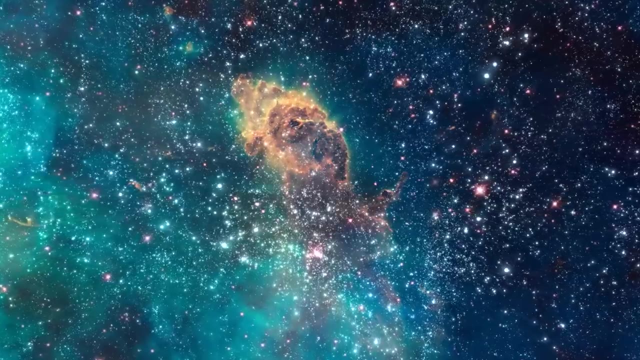 of which there are many different forms, but the underlying idea is to try and get the universe to pick a side, tell us whether there's hidden variables and Einstein's right, or tell us whether truly there is a wave function and that quantum mechanics is real. 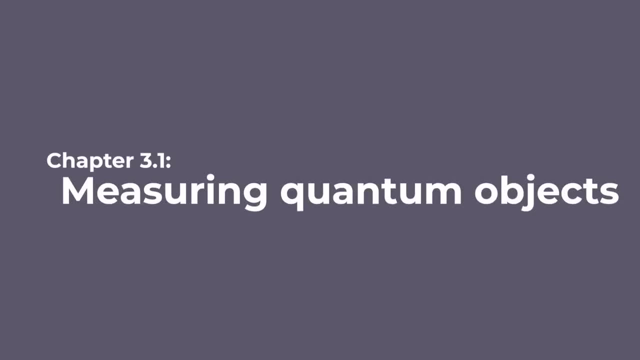 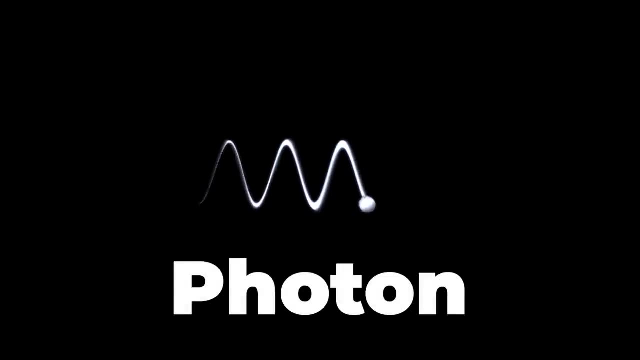 Now this hinges a lot on what happens to quantum objects when you actually go out and measure them. So let me introduce you to the idea for a particle of light called a photon. Photons have a property called polarization, which describes which way the wave of light 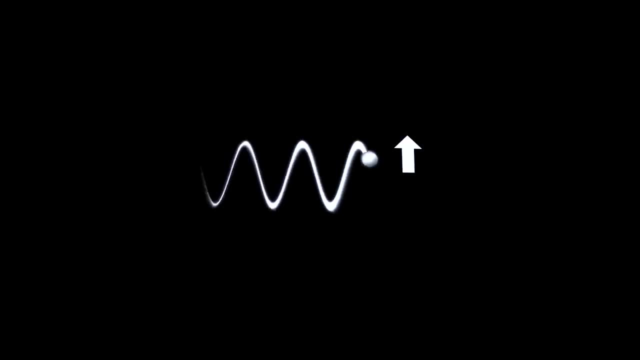 is oscillating through space, either vertically or horizontally, or potentially somewhere in between. If you wanted to measure which state a photon was in, you would put it through a polarizer that lets through either vertical light in one orientation or it will only let through horizontal light. 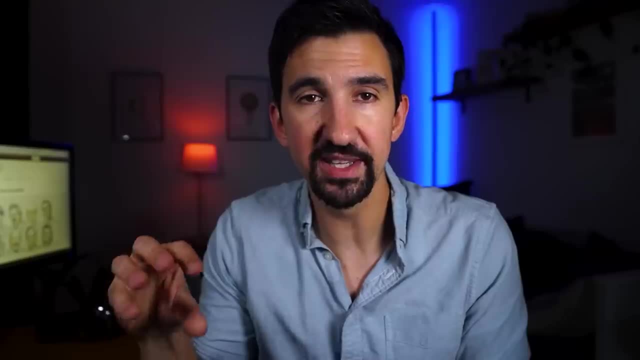 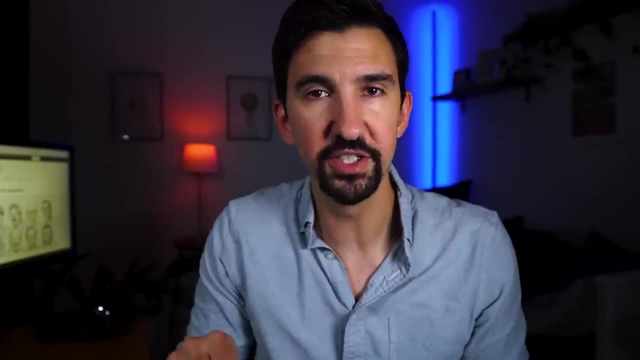 in another orientation. But then at least the detector which you place behind that polarizer knows what sort of light it's detecting. If you fired in randomly polarized light, some of it vertical, some of it horizontal, some of it in between, 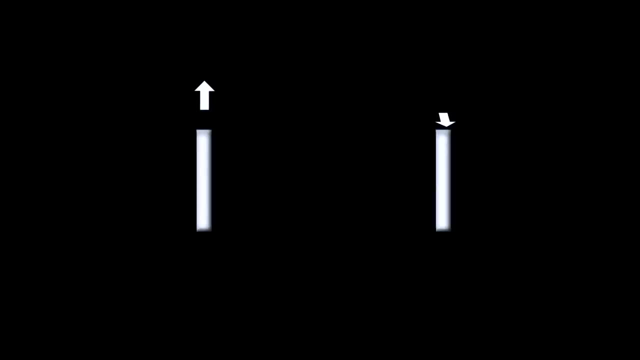 by placing a vertical polarizer first, then a horizontal polarizer after, you would expect correctly to see that no light reached your detector because all polarization angles had been blocked. You can see this effect when using polarizing films, which are the same stuff you find. 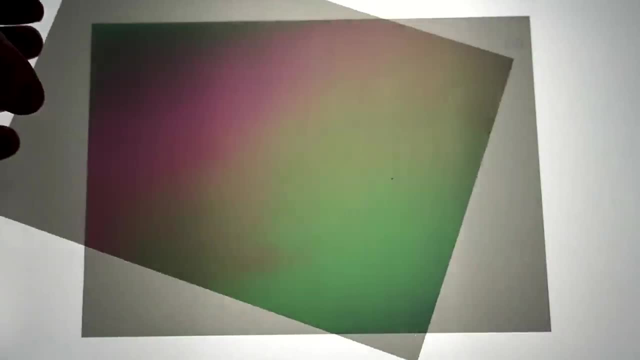 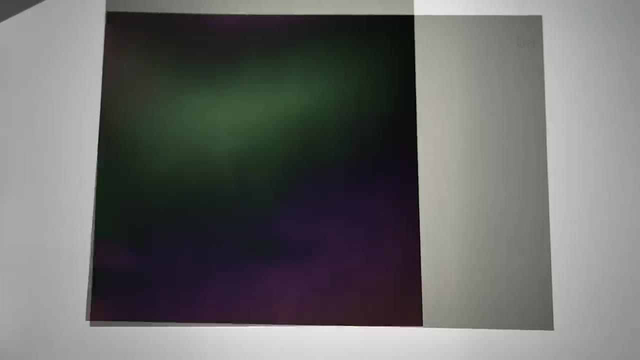 on a pair of polarizing sunglasses. By orienting two polarizing films at 90 degrees to each other, you see no light emerges through them. What is interesting here is that if you place a third polarizer between these two, you suddenly- and, I think, quite counterintuitively- 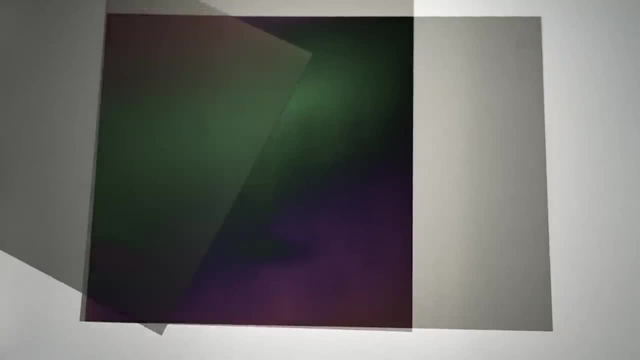 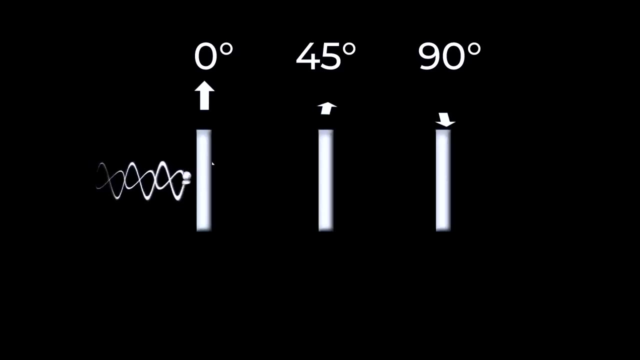 start to see more light. This is because, fundamentally, measuring a particle changes its state, allowing light to slip through the final polarizer, where usually it wouldn't be able to. So you start to see more light than you would otherwise expect. So let's jump back, though, into the story. 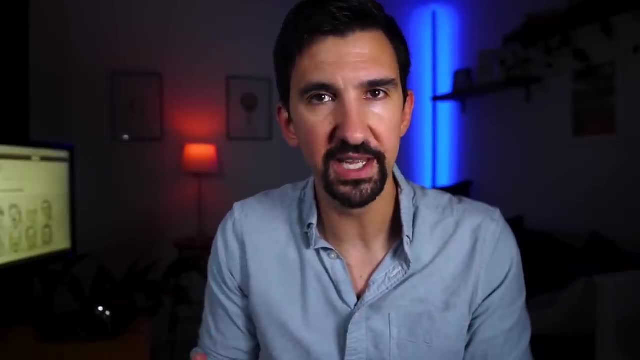 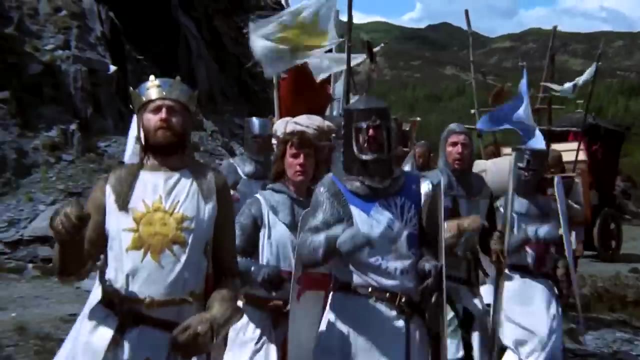 At this point in history, Bell's work was still more theory and thought experiment than anything else, And that, classically, is the problem with theoreticians: If you look at them from a distance, it just looks like a wizard trying to have an argument with you. 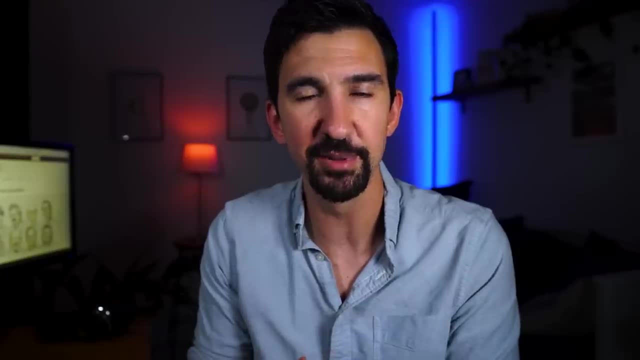 Physicists really needed to find a way of actually completing the experiment, but they couldn't do it, So they had to do a lot of work to make sure that they were able to do it, And that's how they ended up completing an experimental measurement. 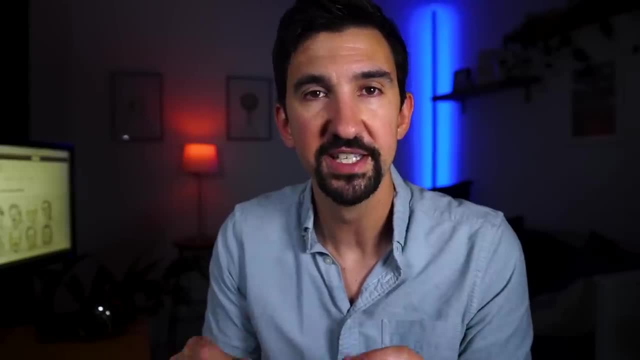 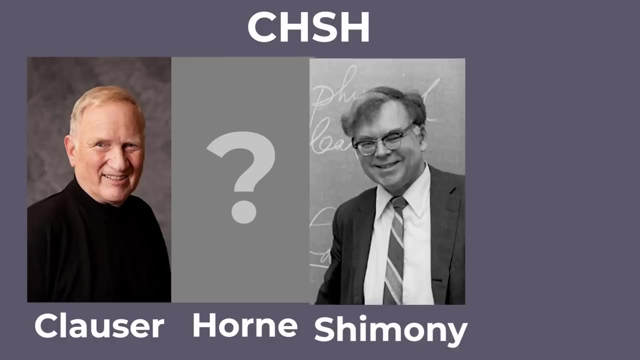 One of the early and most elegant and now heavily evidenced extensions of Bell's theorem work is the CHSH inequality by John Clauser, the Nobel Prize winner that we're talking about here, Michael Horn, Abner Shimony and Richard Holt, And their work here makes this theorem 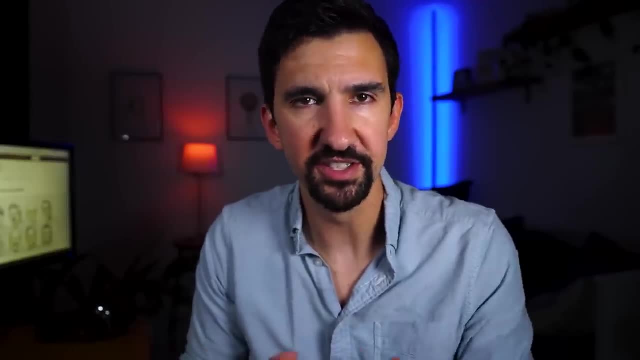 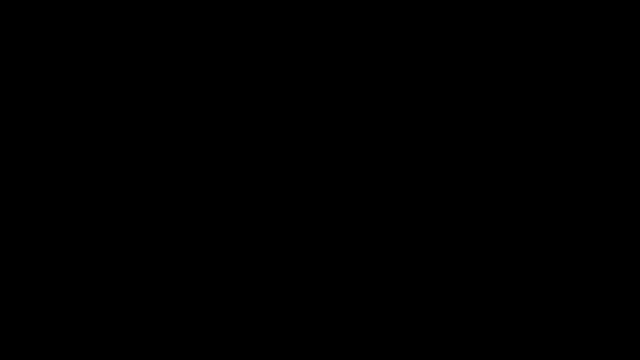 that Bell developed, actually experimentally testable. The scenario they describe is similar to what we talked about before. Two entangled photons are sent in opposite directions to two observers, Alice and Bob. Both Bob and Alice get a polarizer to play with into their setup that helps them determine. 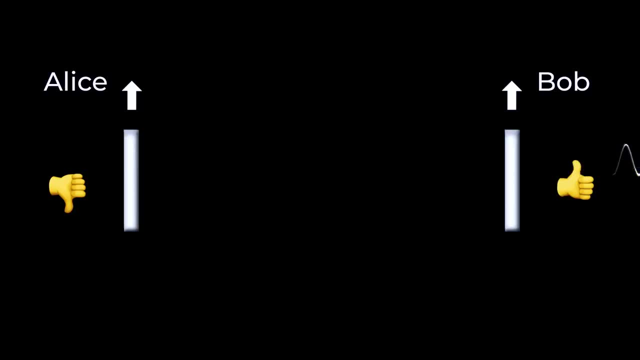 which polarization the light is actually in. And finally, Alice and or Bob at random are told to rotate their polarizers over time and record whether photons arrive successfully or not at their detectors. What we're interested in doing here is counting how frequently that Alice and Bob agree. 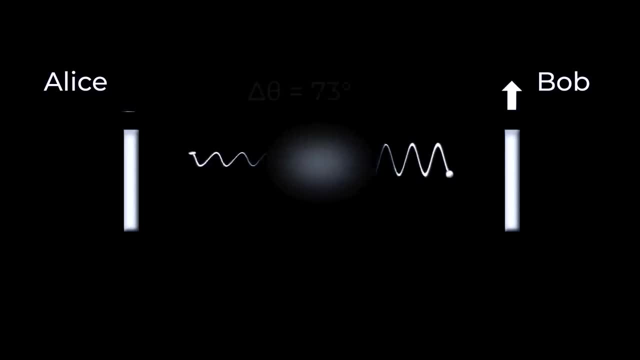 on whether they've seen or not seen a photon. If Alice and Bob perfectly anti-align their polarizers, then they should always both either see a photon or neither one should see a photon. They should always agree on whether photons arrived or photons didn't arrive. 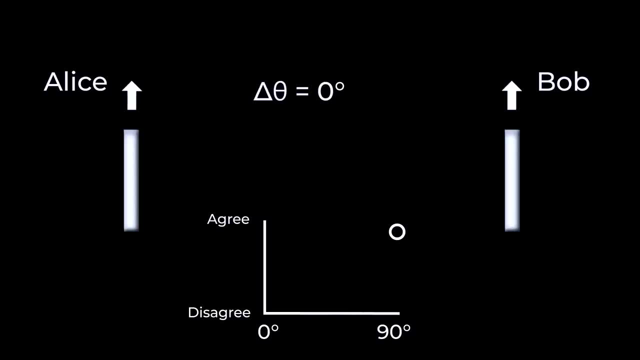 If, however, Alice and Bob both align their polarizers, either Alice should see a photon and Bob shouldn't see one, or Bob should see a photon and Alice shouldn't see one. The interesting part happens at angles between these positions. If the universe is real and photons are truly independent, 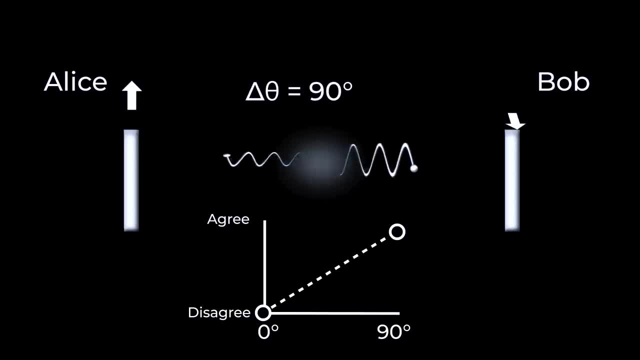 Alice and Bob's rate of agreement should linearly move between full agreement and full disagreement. If, however, the universe is not real, we should expect to see a higher rate of coincidence than otherwise expected, just like in our three polarizer setup. 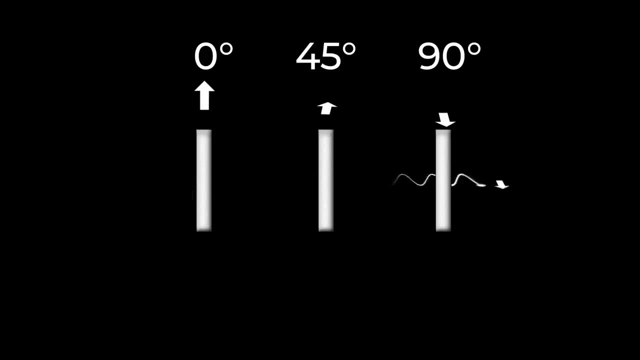 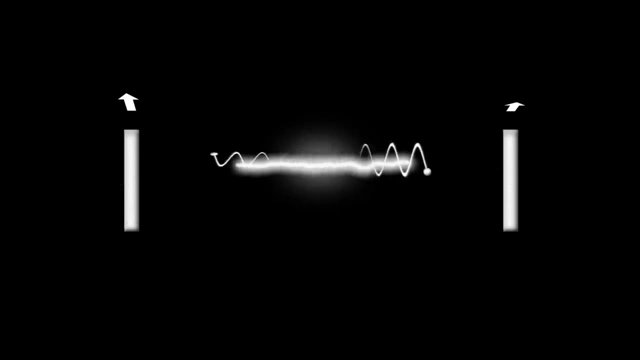 except now our polarizers are on the other side of the universe from each other, and the same photon isn't going through both, Or is it? This can only be true if the particles are really still connected to let each other know which polarization state to be in. 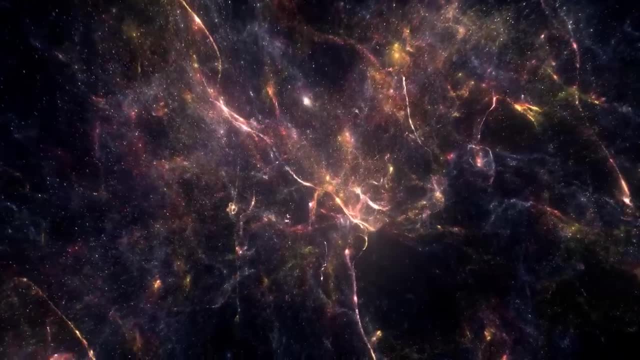 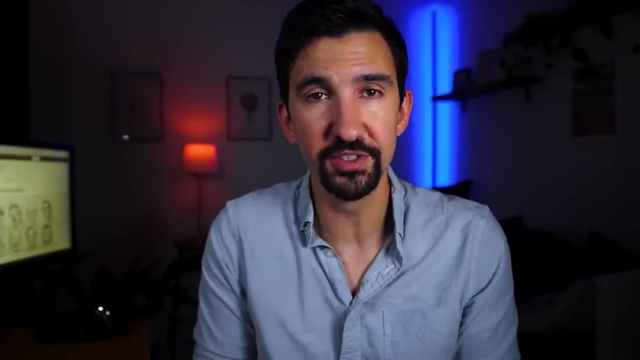 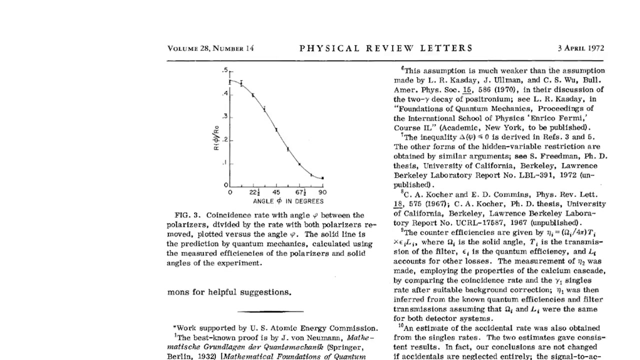 so that measurement on one truly does affect measurement on the other. And in 1972, it was John Clauser who built the first experimental setup capable of conducting this measurement. In the paper that he released that year, this was the figure that he displayed. 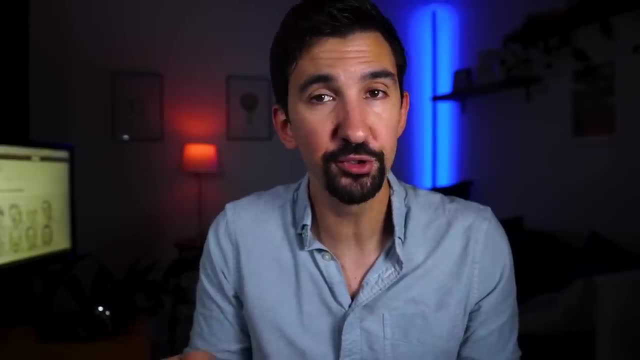 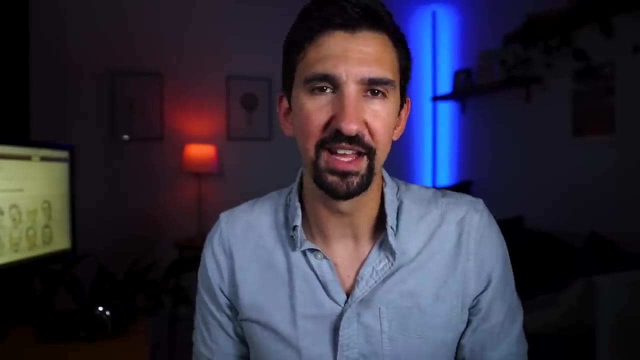 exactly matching the prediction of quantum mechanics, Proving that the universe isn't locally real, that Einstein's deterministic view was incorrect And the story from this point goes- I'm not sure if it really happened or not- that excited by proving the result. 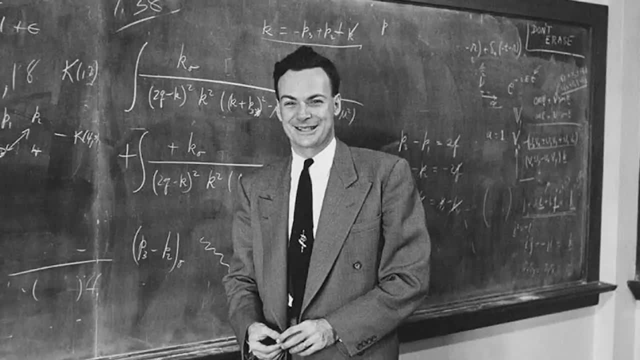 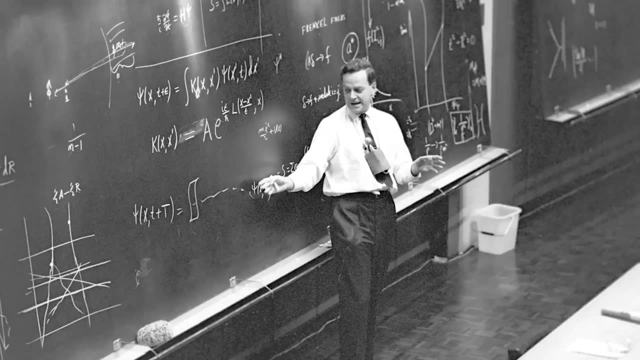 Clauser runs into Richard Feynman's office to tell him the news And, in classic Feynman fashion, Feynman throws him out of his office, forever doubting quantum mechanics, and tells him: good, now get on with some real physics. 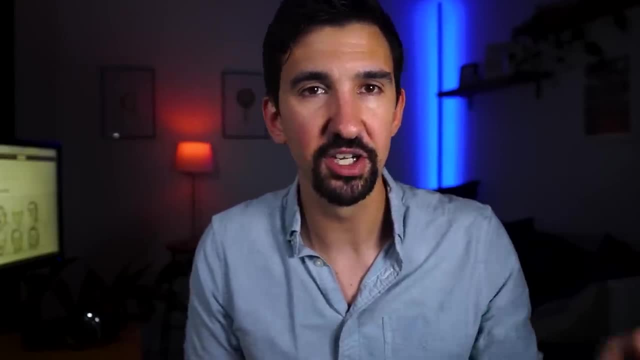 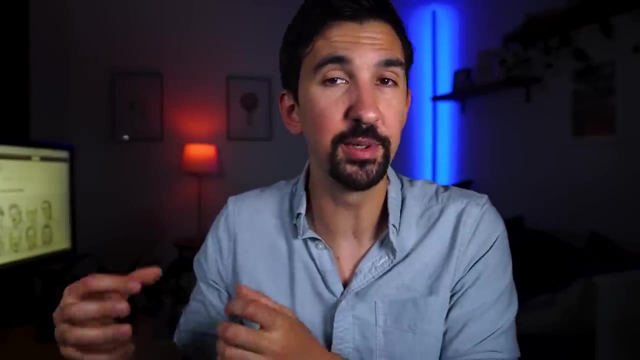 The other Nobel Prize recipients, Elaine Aspect and Anton Zalinger, closed important loopholes that remained within this experiment, as well as showing that quantum entanglement can be transferred to other particles in a process called quantum teleportation. All this to say that, without a doubt,